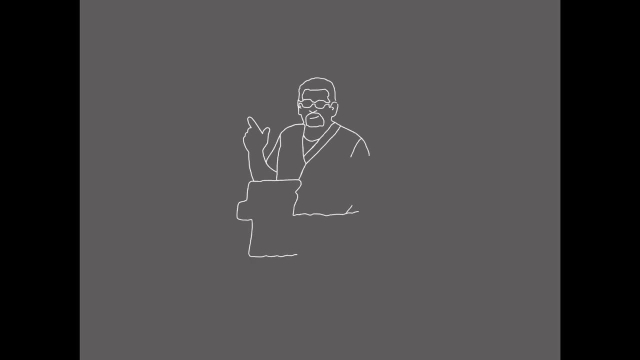 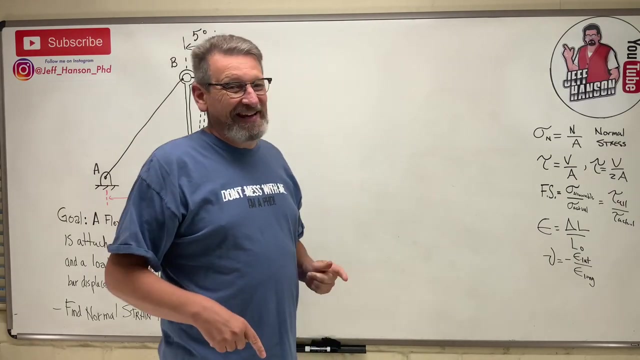 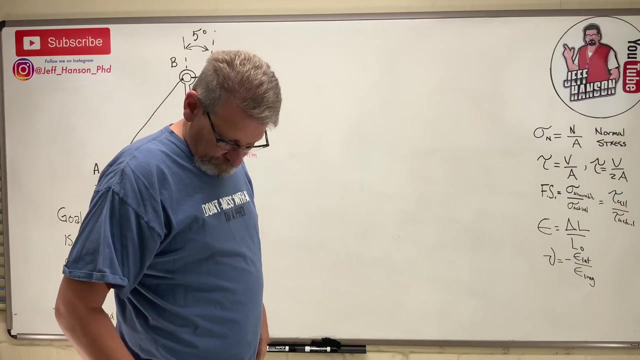 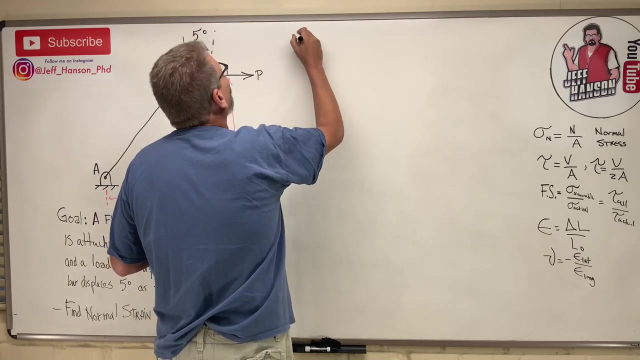 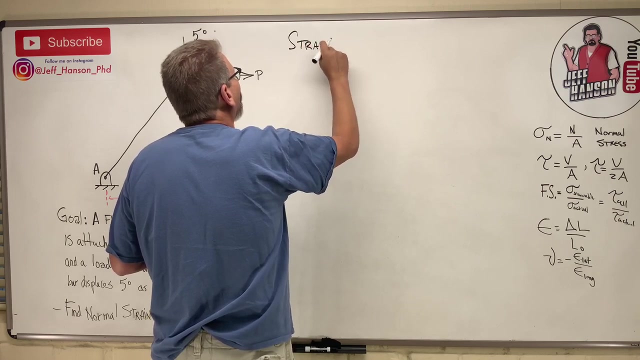 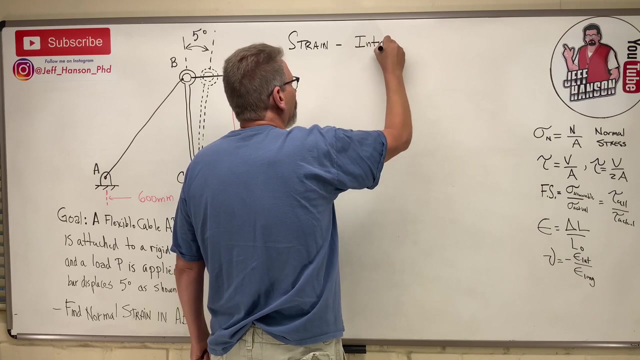 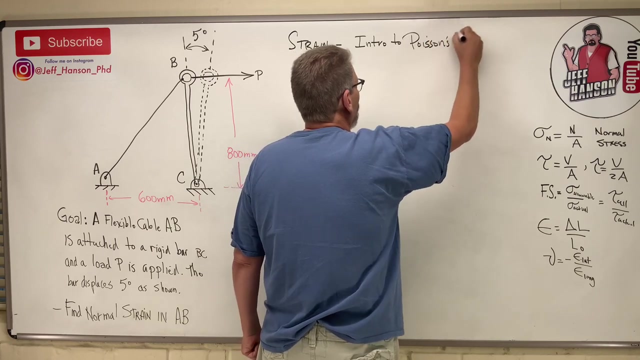 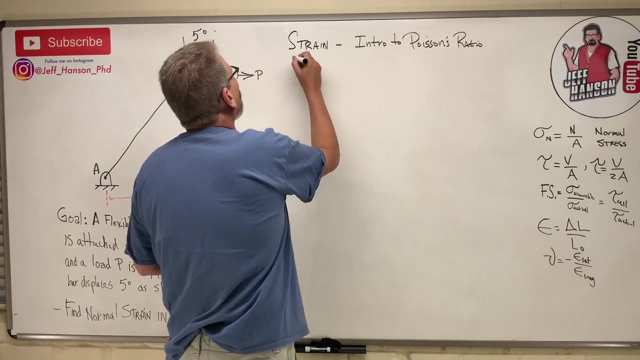 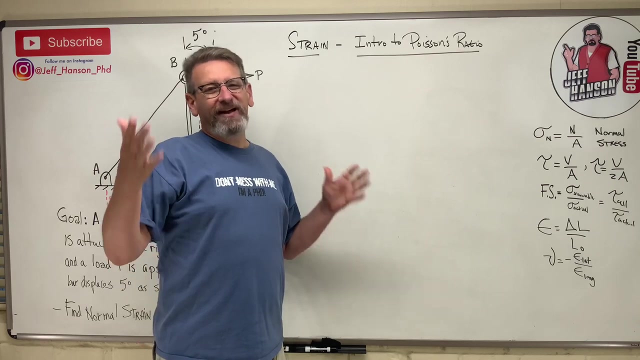 All right people, welcome back. We're talking about strain today. It's the next section of the book. All right, let me write it on the board. All right, let me write it on the board. All right, let me write it on the board. 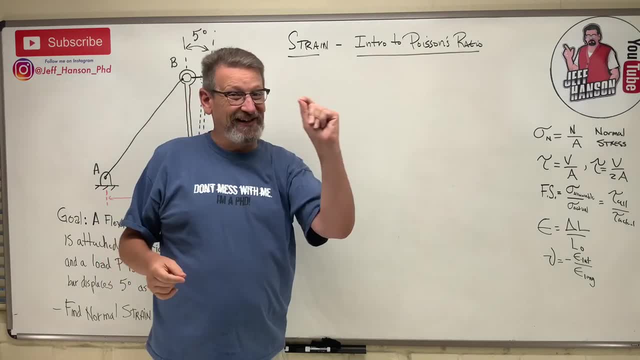 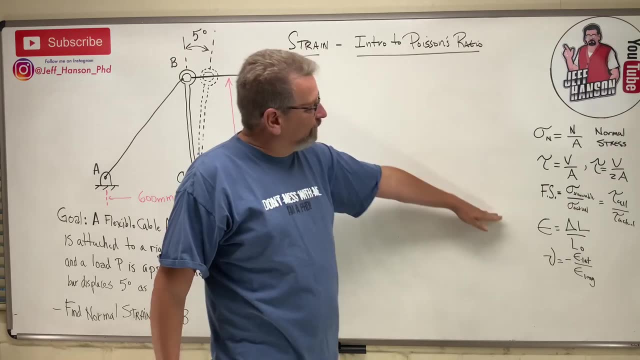 All right, today we're talking about strain and an introduction to Poisson's ratio, So let's start talking about strain. We're going to talk about strain primarily today. okay, We have some new equations on our equation sheet that we've been adding up over here as we go along our videos. 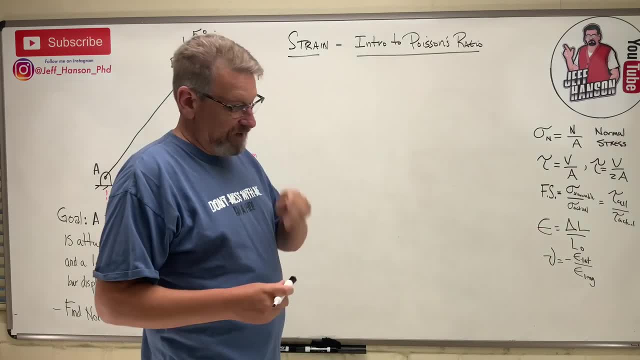 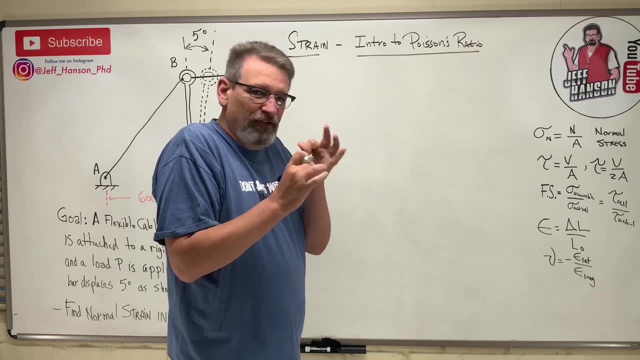 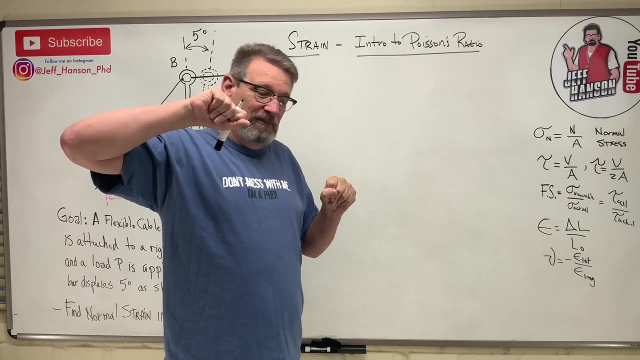 And here is strain. So what is strain? We know what stress is. Stress is like the intensity of a force, how intense it is on a certain area. right, Strain is just Strain is just deformation. As I pull on something, it elongates, It gets longer, It stretches, right. 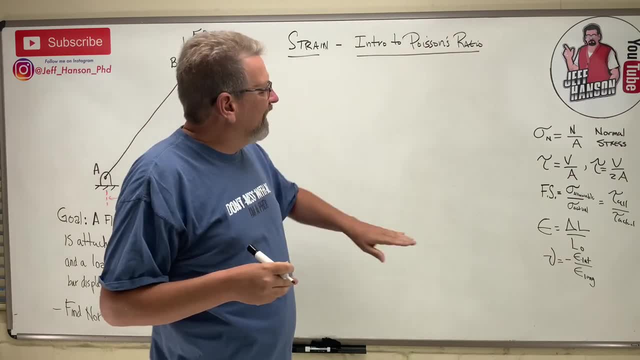 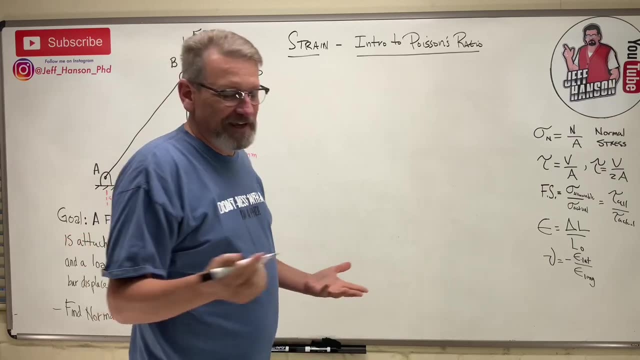 That's strain, And so there's an equation for strain. Strain is given with the Greek letter epsilon. okay, My students call it circle E. I don't you know. come on, circle E. There you go. there's circle E. 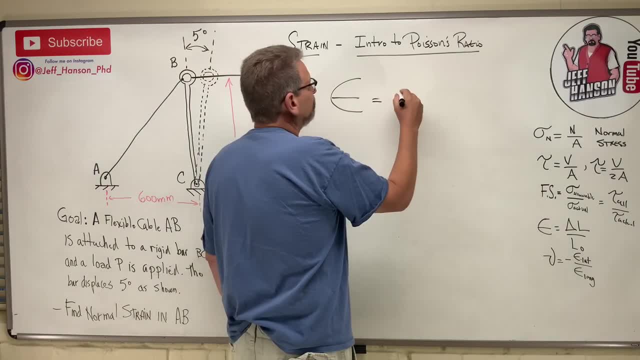 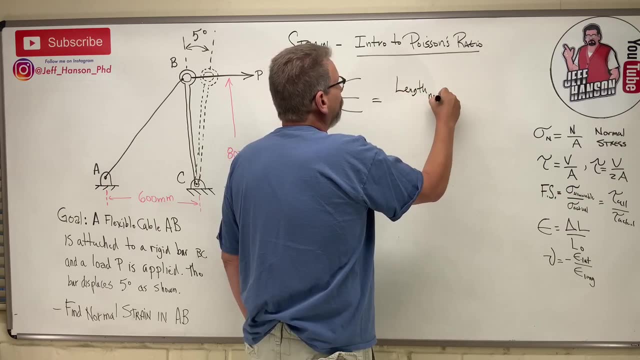 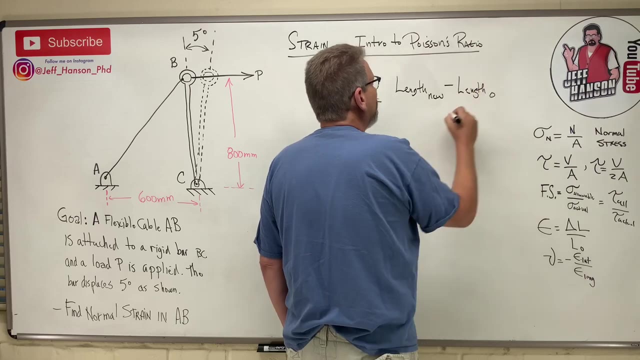 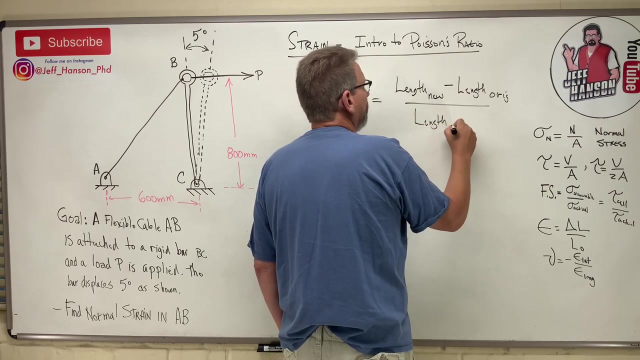 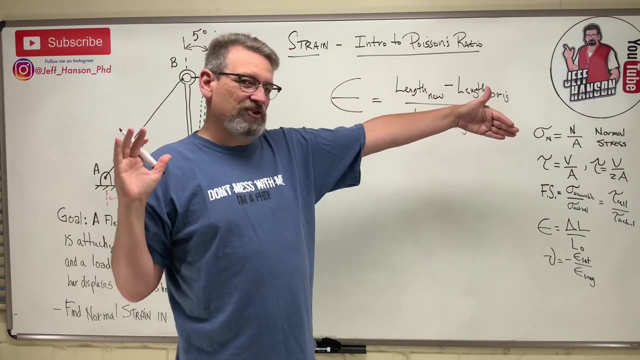 And epsilon is the length of something, The new length, like the stretched length, minus the length original divided by original, by length original. Okay, So take the new length, take the overall length that the thing is stretched after you put a little force on it, right? 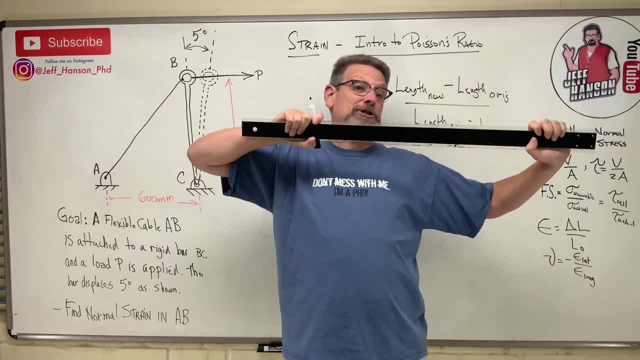 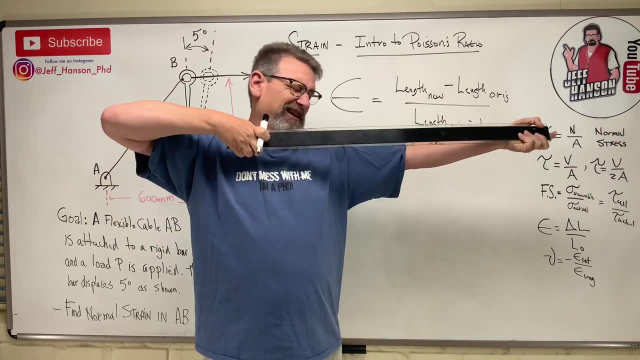 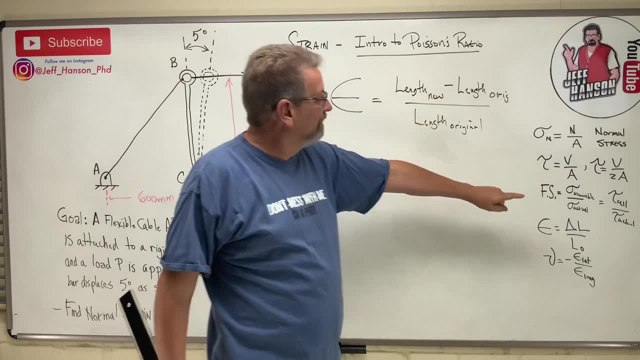 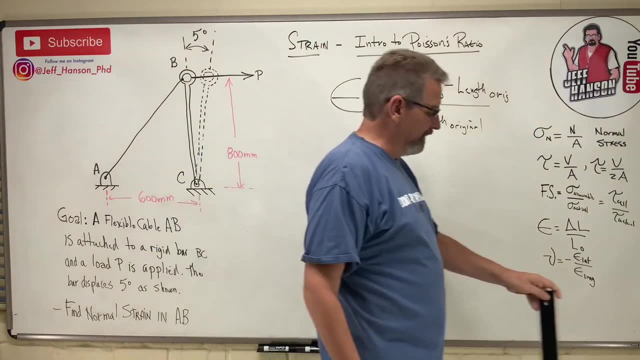 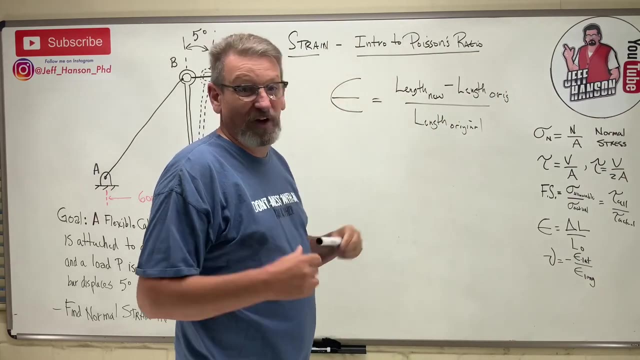 So subtract the original length from the new length, That leaves me the change in length, the delta L, And then divide that by the original length. Now the units on this are a little weird, Not too weird In that length is in inches and this is in inches as well. 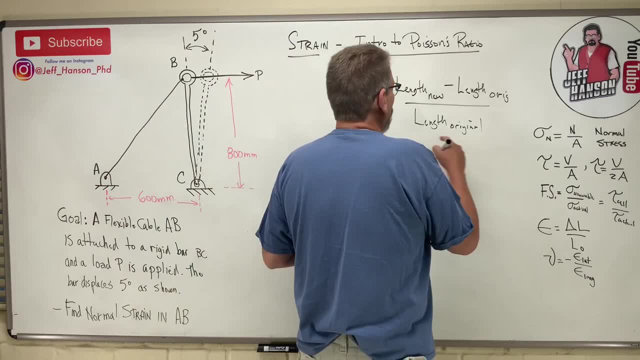 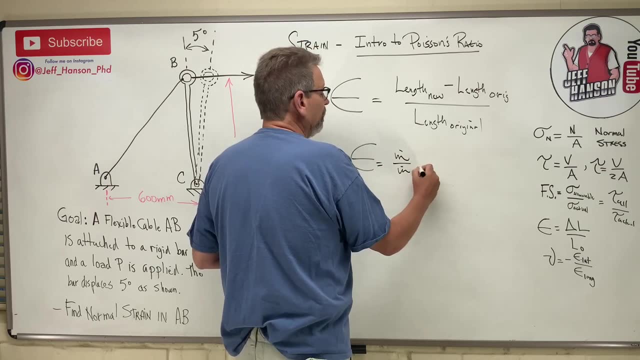 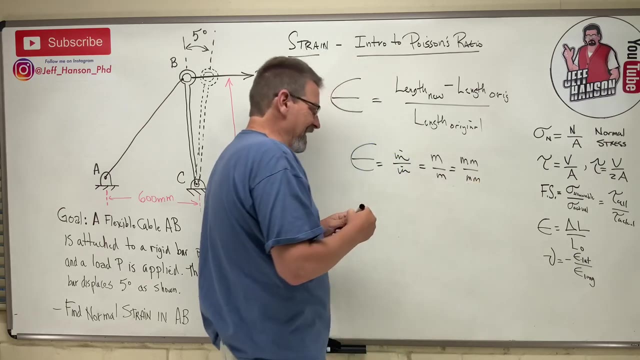 Or meters and meters, if you're a metric guy, right. So the units- Units for strain- are in inches per inch or meters per meter or millimeter per millimeter. right Now. those really cancel out, so you could think of it as kind of a unit-less thing. 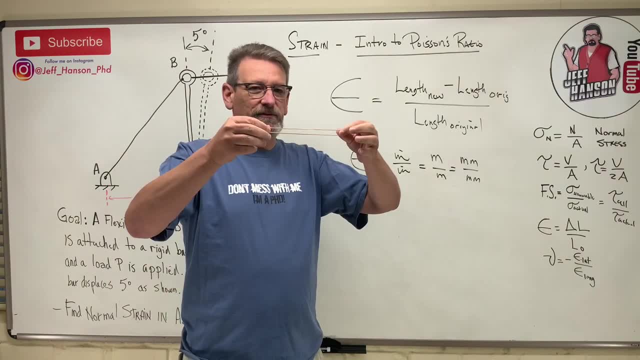 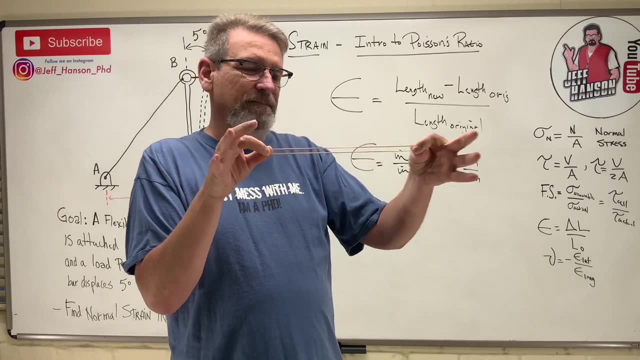 But let's say I had something like this, a rubber band. okay, So this is my beam. let's say, Okay, So as I start putting a force on this beam it starts to stretch. Now, that's about as far as I want to stretch that right. 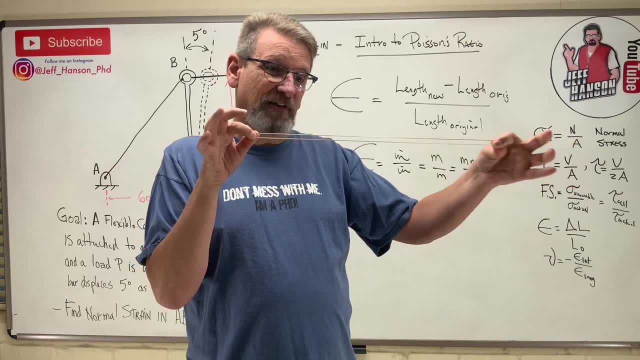 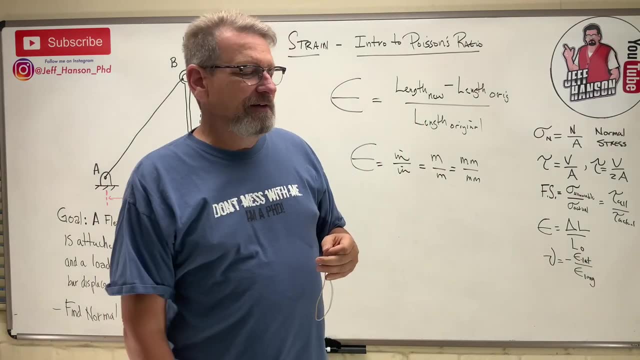 So if I measured that new length and divided that by, Or that you know, subtracted the original length and then divided it by the original length, I would have strain Now inches per inch. what does that mean? Well, look, how many inches of this rubber band do I have? 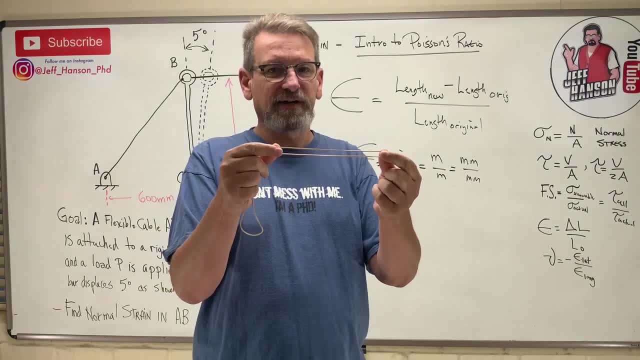 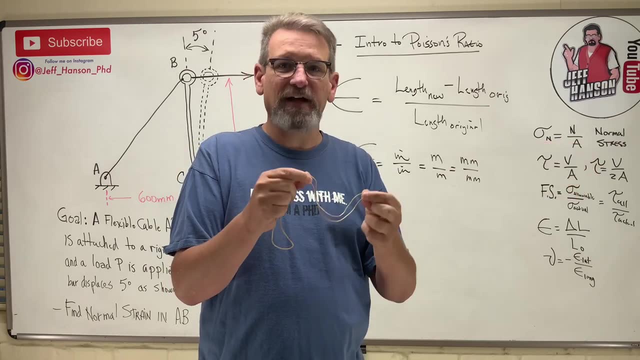 Let's say that's- I don't know- looks like about 7 inches right, And when I stretch it, that looks like about 20 inches. Let's say 21.. 21 inches right. It got three times longer. 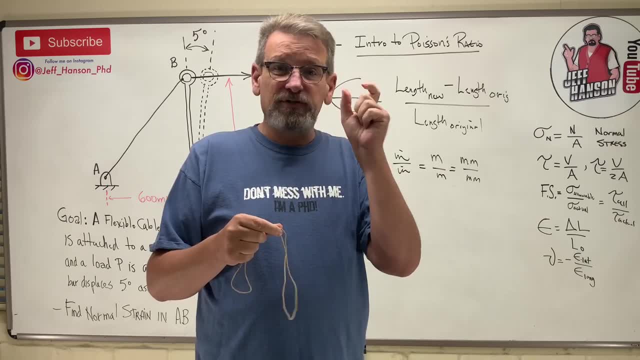 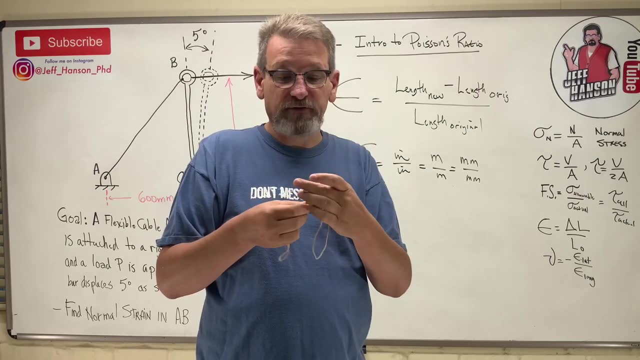 So for every inch of rubber band it stretched 3 inches long. right, That's inches per inch. So what if? what if I have more inches of rubber band? What's going to happen? Let me just make this rubber band longer, okay? 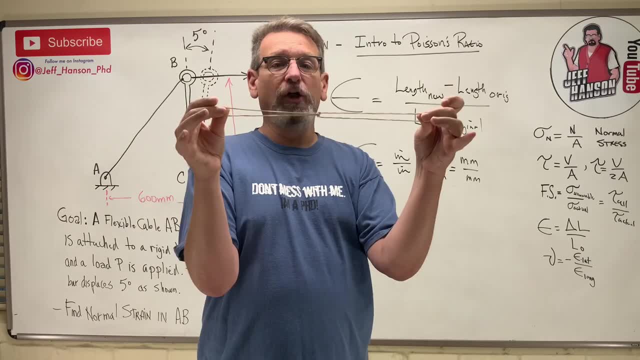 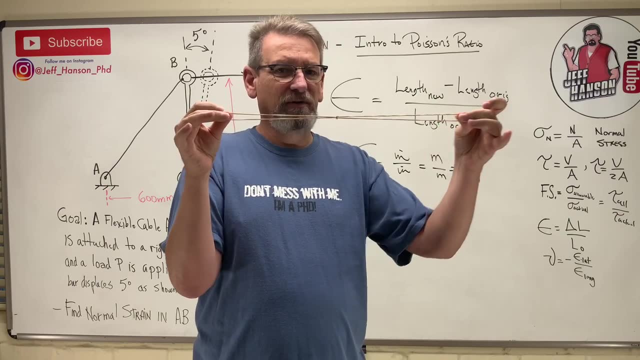 Now the rubber band is that long unstretched? okay, It's twice as long, It's 14 inches long now. So how long is this going to be able to stretch? now, Right, And inches per inch. oh, that's about as far. right, there is about as far as we'll go. 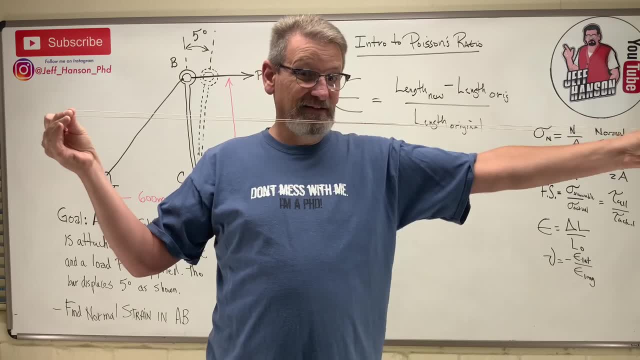 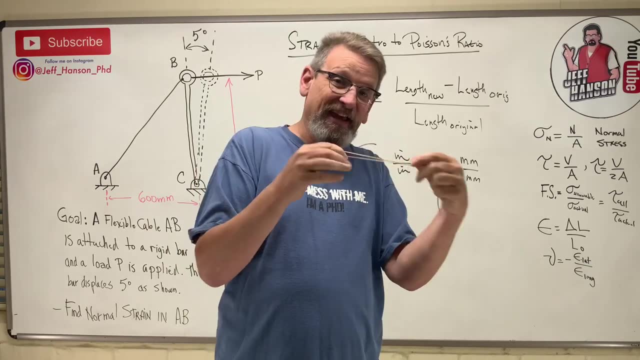 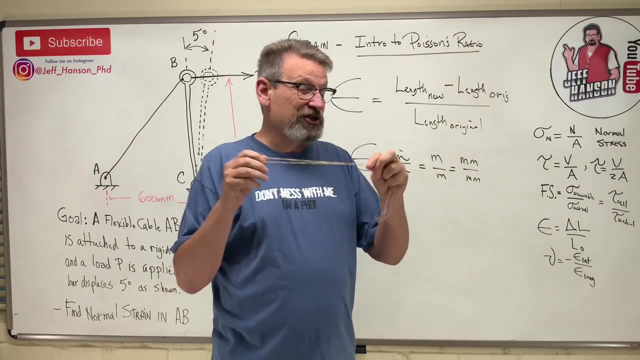 I bet you that's about 42 inches, right? So I had more inches of rubber band. So if each inch stretches so many inches, right, the more inches of it you have, the more stretch you get, And that's what that kind of means. when you say inches per inch, it's like how many inches? 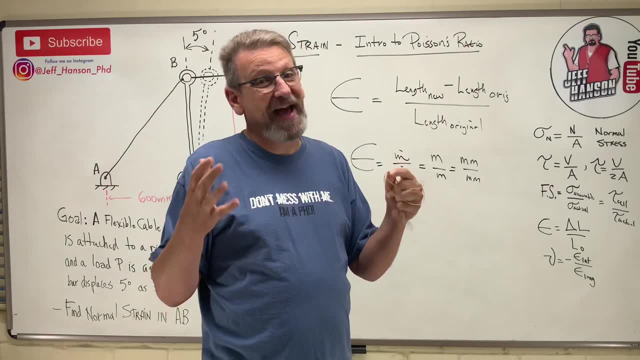 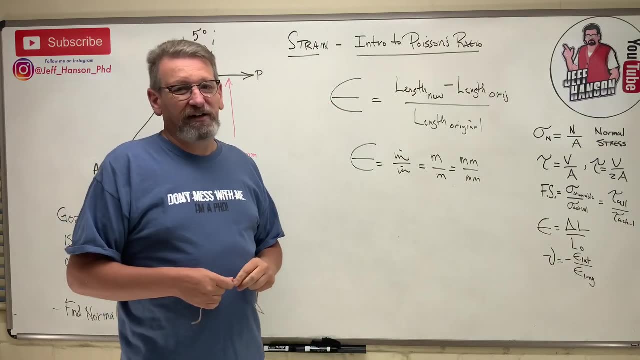 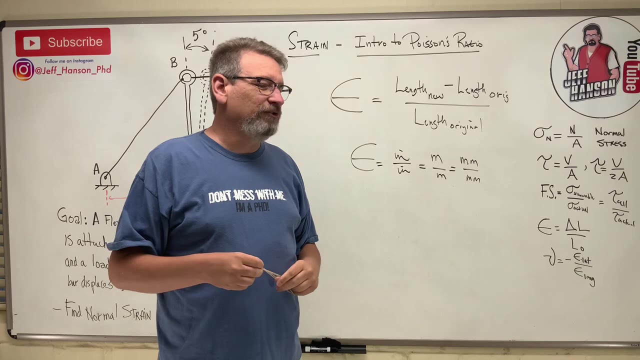 does it stretch for each inch of material that you have, or each millimeter of material that you have? So that is deformation. It is strain, okay, And this, of course, is axial. There is some other kind of strain we're going to talk about, but most of the deformation. 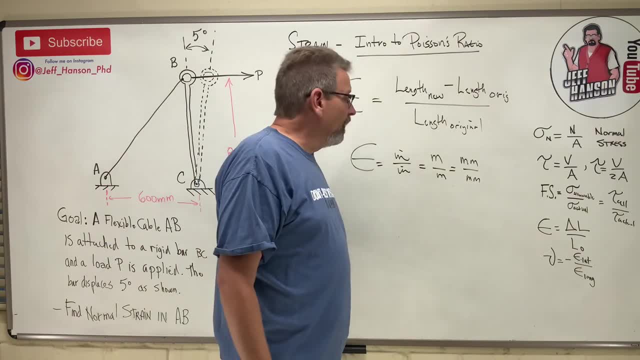 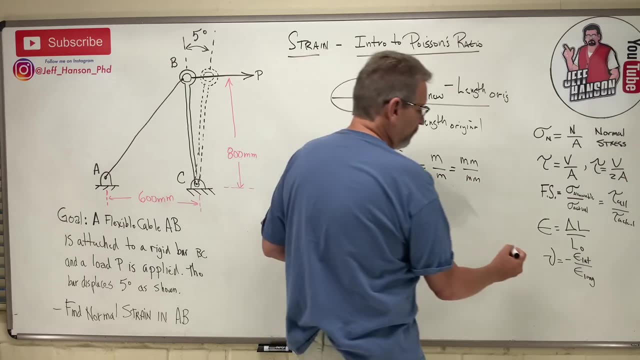 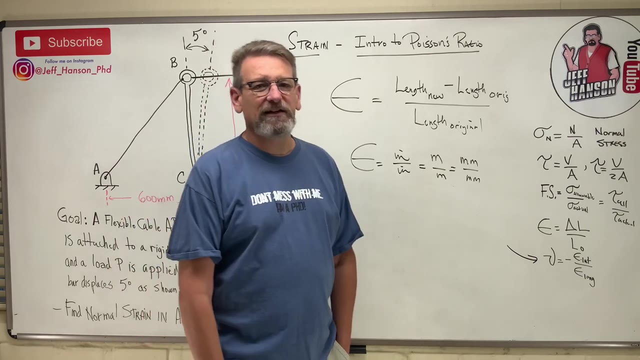 is going to be axial. Now, another, another thing that you'll see here when you're talking about strain problems, is this guy down here, which is Poisson's ratio. okay, And Poisson's ratio. I like to think of it as you know it's going to be, you know. 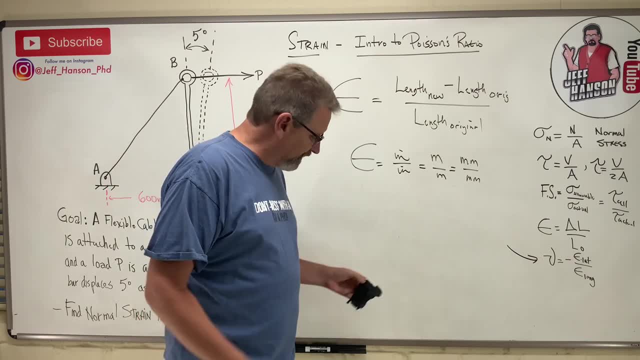 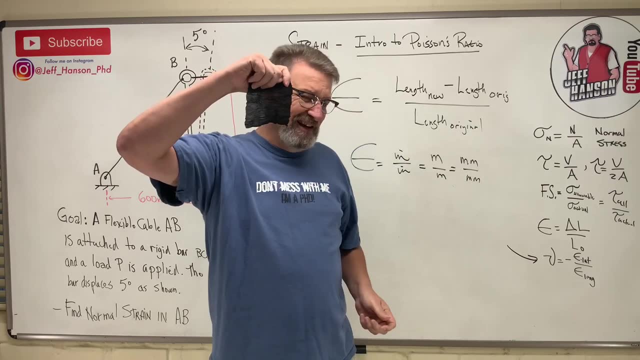 as the Stay Puft Marshmallow Rule Here. let me, I've got a little piece of stretchy material here, okay, So I've got a little square of stretchy material. If I elongate this material, what's going to happen? 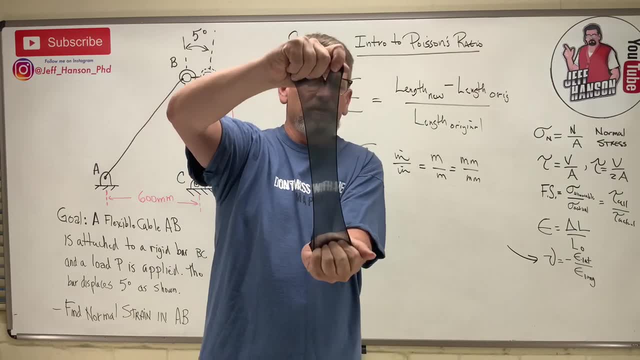 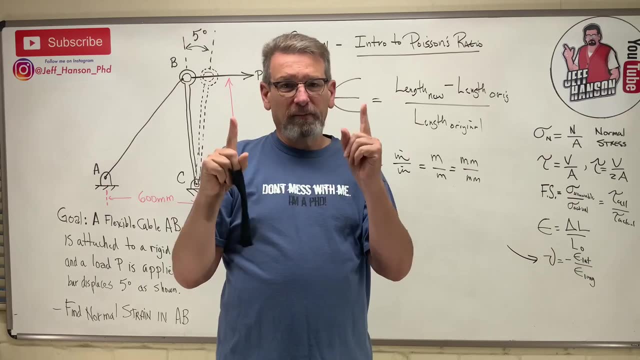 So what's the width of the material? As I start to stretch the material, what happens to the width of the material? okay, It reduces, doesn't it? It goes from that wide to this wide, So, and that's what's called Poisson's ratio. 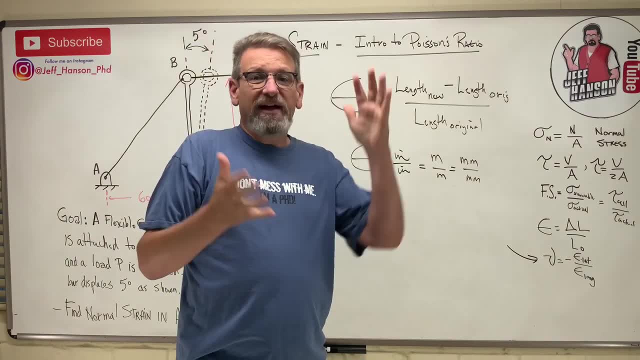 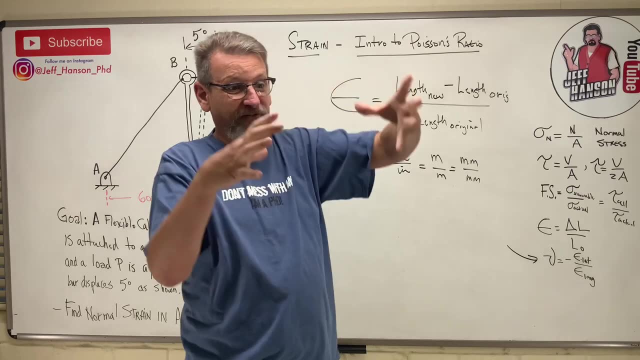 As I stretch something, it gets narrower. As I compress something, it's going to get wider. I like to think of it as the Stay Puft Marshmallow Rule. right, If you had a big, giant fat marshmallow and you squeeze that marshmallow, what's going? 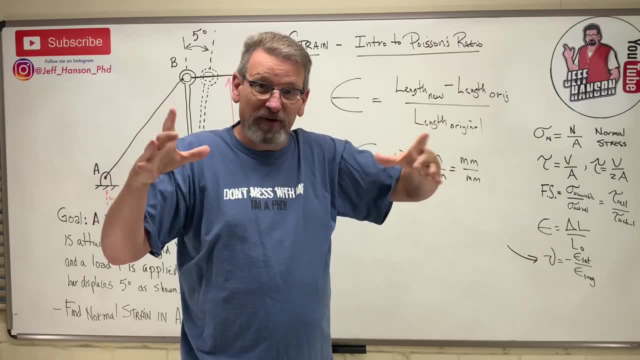 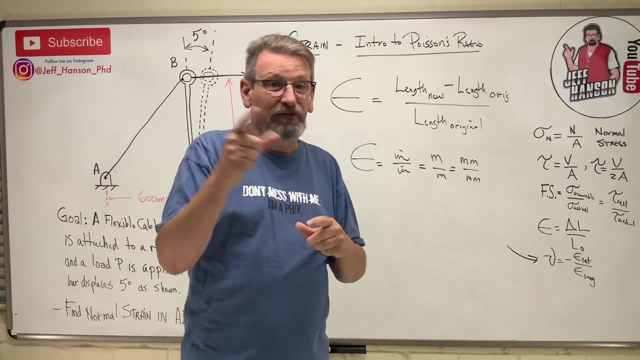 to happen to it. Right, It's going to get bigger. on the diameter, The ratio of how much it shrinks laterally or longitudinally to laterally is Poisson's ratio. okay, And here's the equation for that. 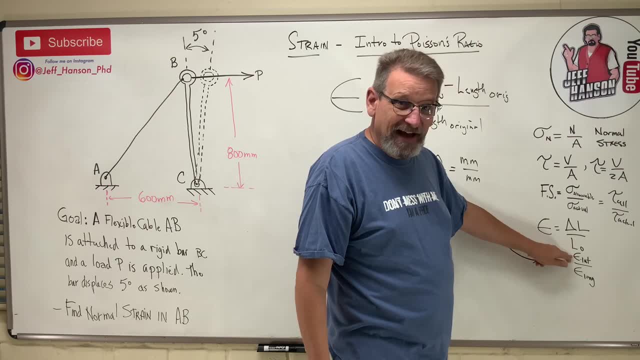 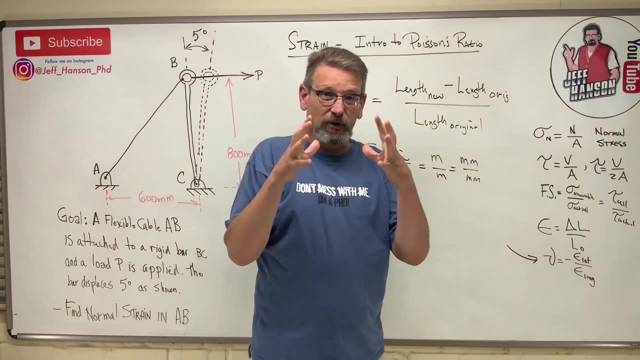 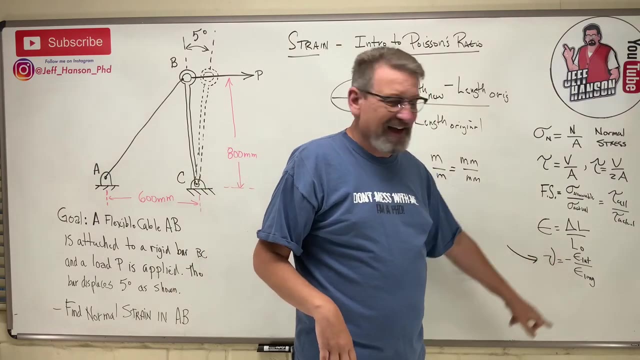 So Poisson's ratio is Strain lateral divided by strain longitudinal. So longitudinal would be along the axis right, And so lateral would be that cross dimension there. Okay. So why is it negative? Why is there a negative there? Okay, 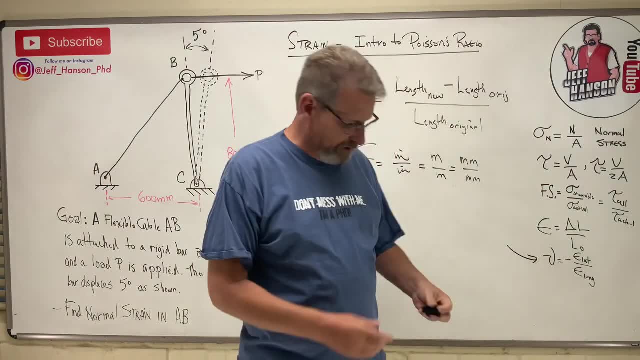 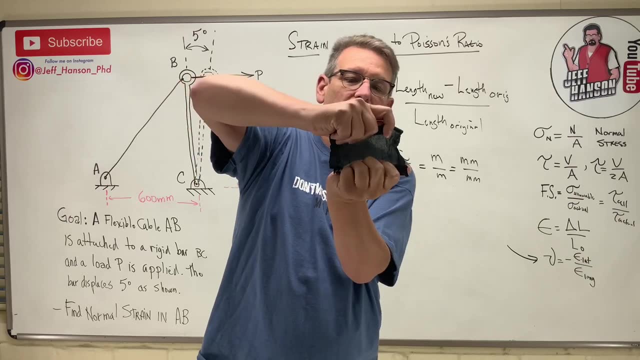 So imagine my little piece of material. Where's my little piece of Here? it is right here, okay, My little piece of material, okay. So as I stretch it, you know, axially, Longitudinally, that dimension is getting bigger. 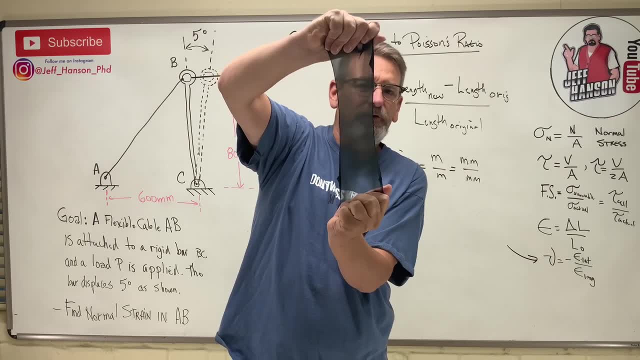 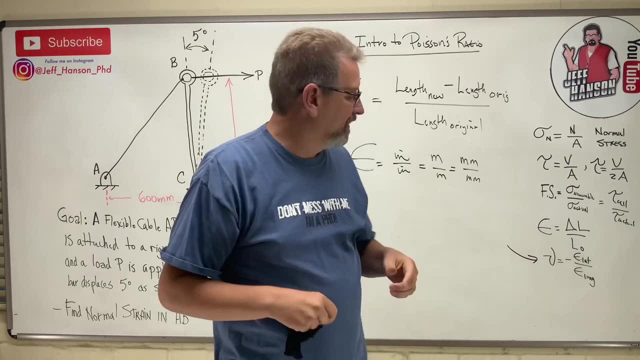 That's a positive sign. But what's happening in the lateral direction? It's getting narrower. That's a negative, isn't it? It's shrinking in dimension. So that negative sign right there. So, because a positive divided by a negative right gives you a negative, 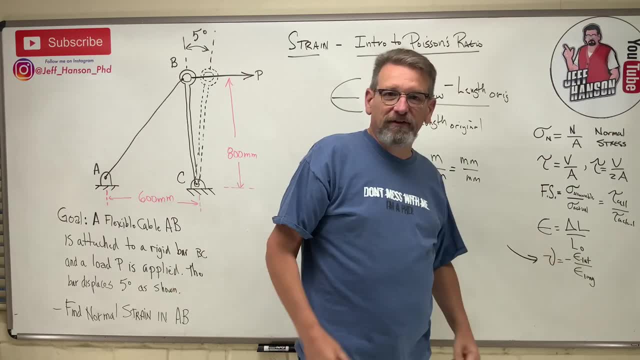 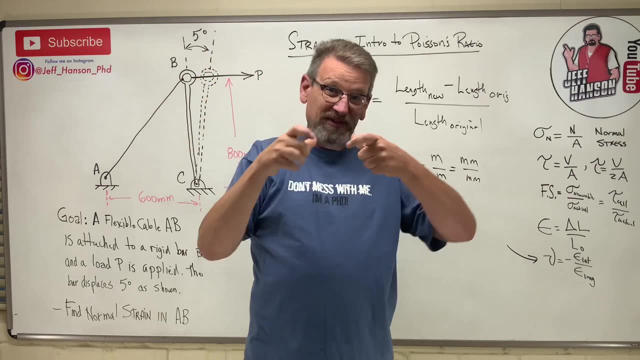 And then what does this negative do? It flips it back to a positive And same thing. If I compress it right, If I compress it, the longitudinal is getting smaller, But the lateral is getting bigger. So there's always One of them is always negative. 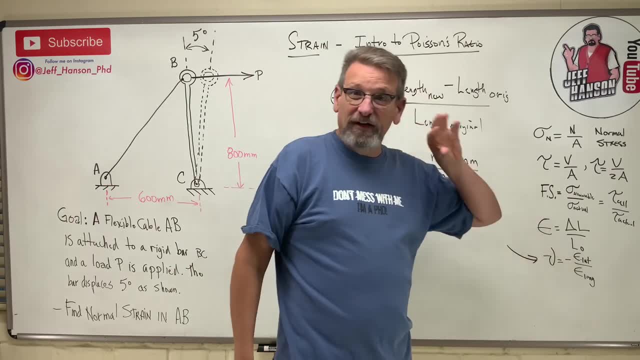 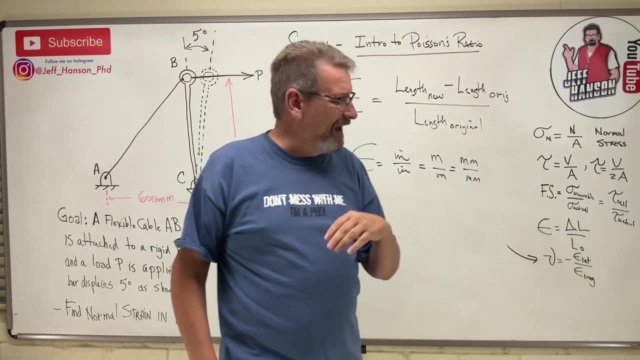 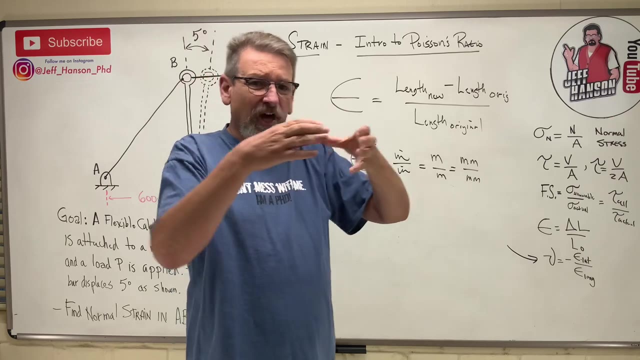 One of them is always positive And that negative sign flips it back, so that Poisson's ratio is always a positive number. So Poisson's ratio is between 0 and 0.5.. Can you think of a material that as you compress it maybe doesn't grow, like we're talking about? 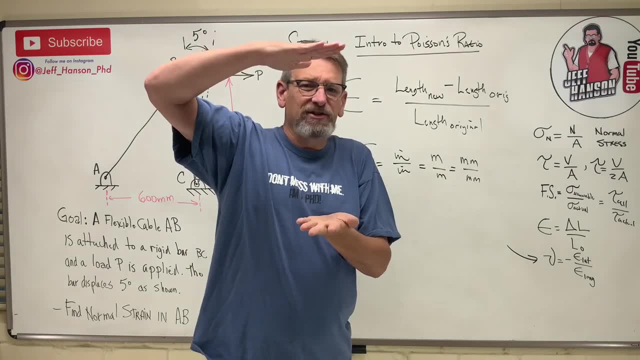 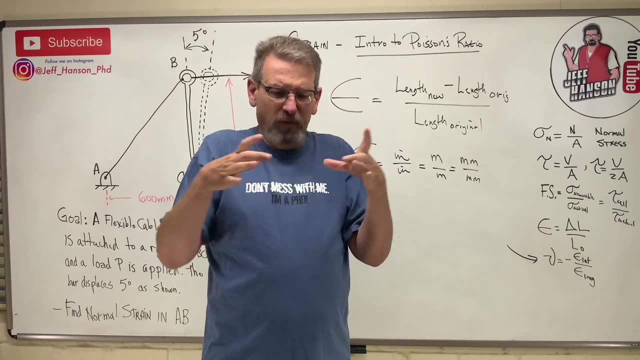 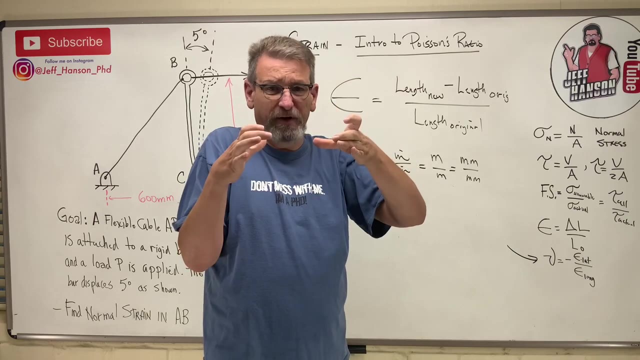 How about something like cork right? A lot of air is entrained in cork Right. So as I compress that, those pockets of air will compress, right, But it won't necessarily grow in the diameter. But something like rubber. you know, if I compress it an inch it gets bigger, almost an inch right? 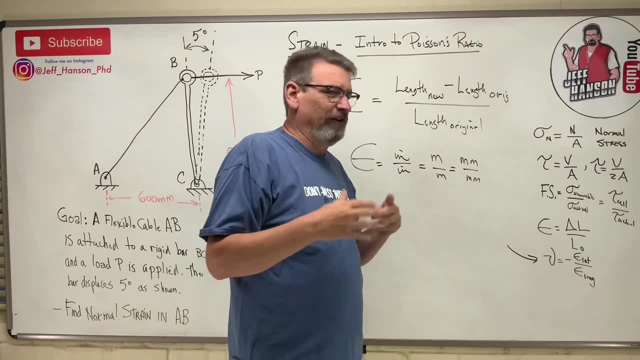 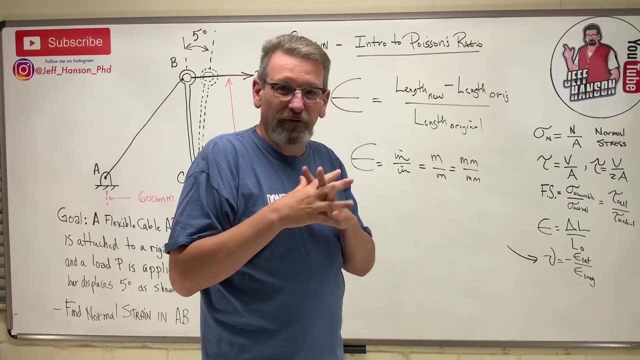 So that's kind of the spectrum between different materials. Aluminum is like 0.29 for Poisson's ratio, Steel 0.27 to 0.30, depending on which flavor of steel you're talking about- And so Poisson's ratio. again, that's what we're talking about. 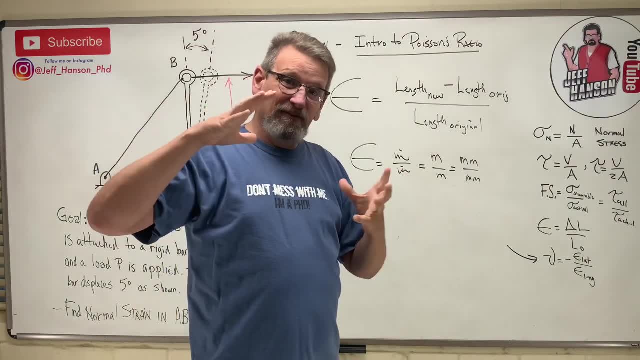 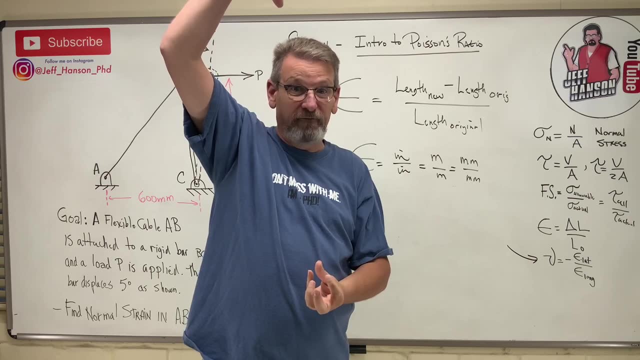 We're talking about today. As I stretch something, right, it gets smaller in diameter Because you think of it, there's only so many molecules in there, right? And if I make that thing longer, those molecules got to come from somewhere. 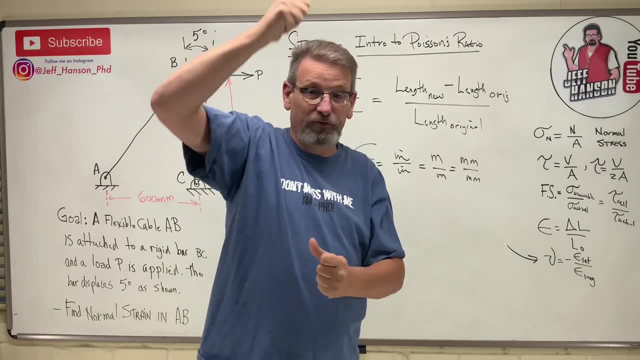 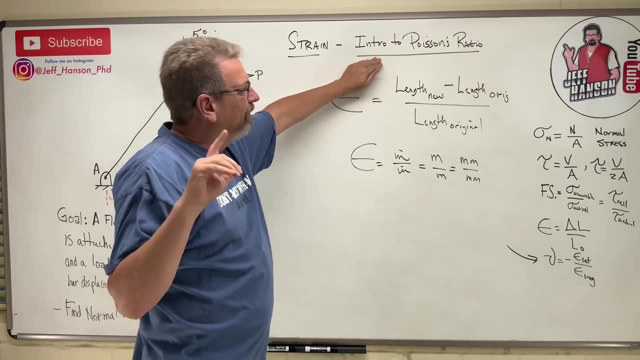 Where do they come from? From the radius right. You know they're all changing places, aren't they? So that's Poisson's ratio. I'm not going to work that in our problem today, But we'll have a sample problem on Poisson's ratio, not to worry. 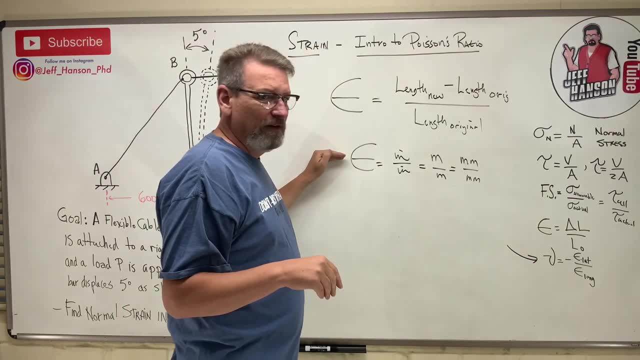 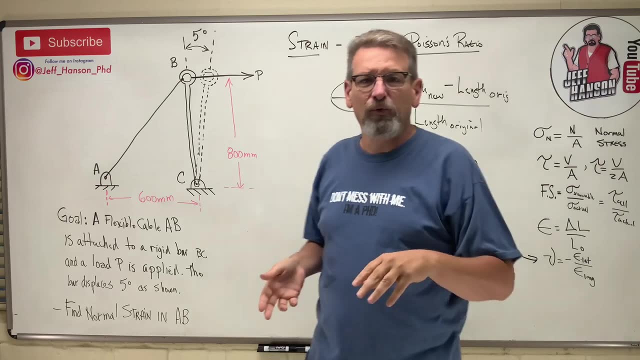 But now it's very closely tied with Strain, with deformation, okay, So now you understand what Poisson's ratio is. It's the Stay Puft Marshmallow rule, man, And you know Poisson. Poisson is French for fish, you know. 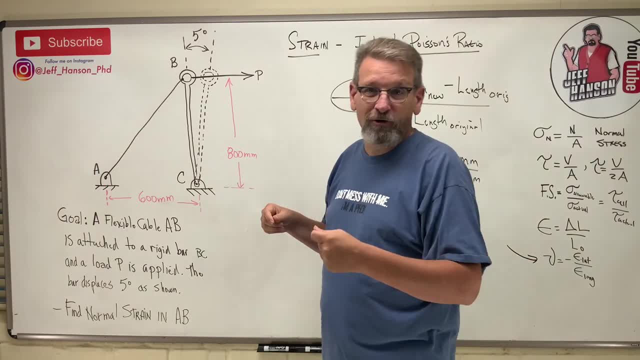 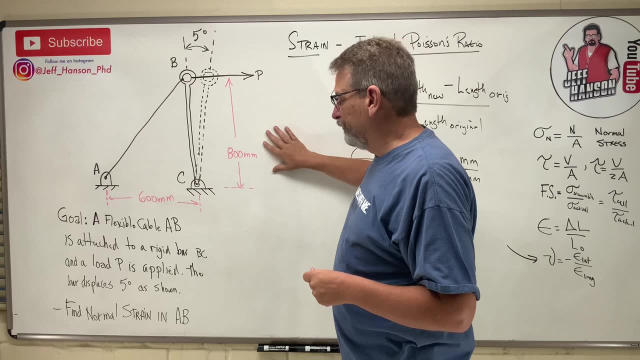 He was a French guy, He had a curly mustache and he went Ha ha ha Because, Oh that's, I'm sorry, I apologize, French people. Okay, here we go. Next, let's work this little sample problem here. 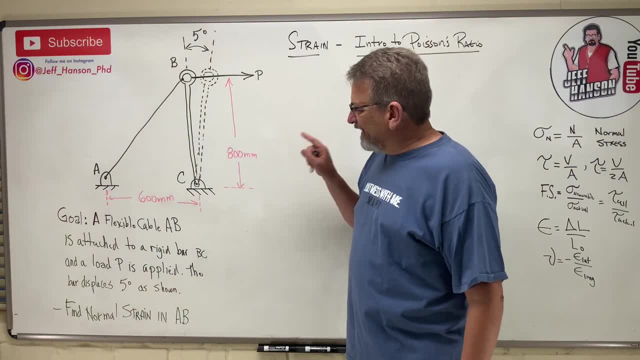 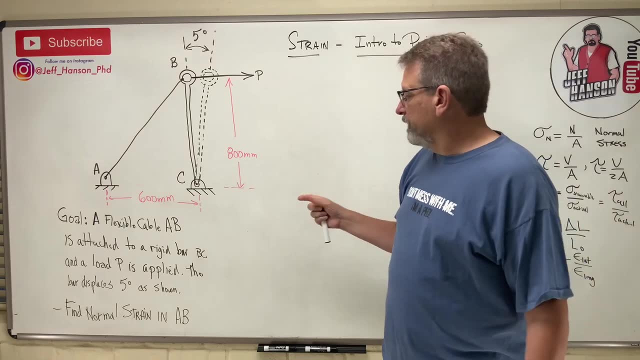 Let me erase my board and work this. All right. for this problem they say a flexible cable AB- That's here Now. flexible just means that it'll stretch right- Is attached to a rigid bar BC. Here's the rigid bar. 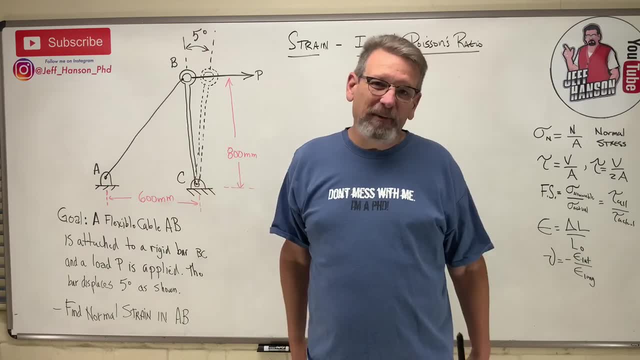 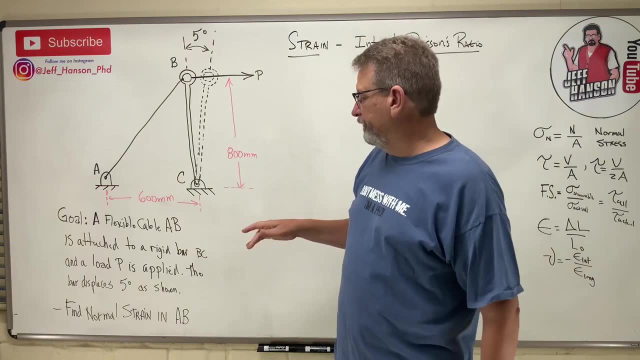 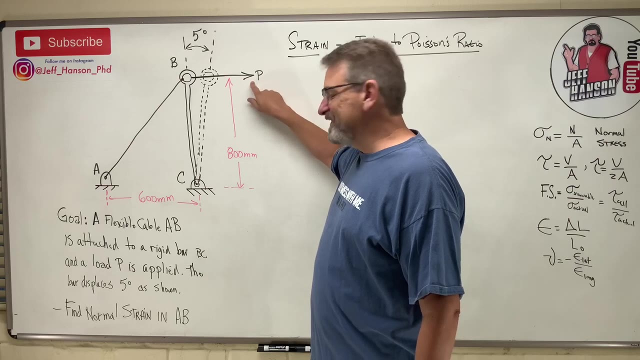 The word rigid means it's magic, It doesn't bend, It doesn't deflect. Really, all bars bend and deflect, But in solid. sometimes we'll have magic rigid ones, okay, And a load P is applied here And the bar displaces five degrees. 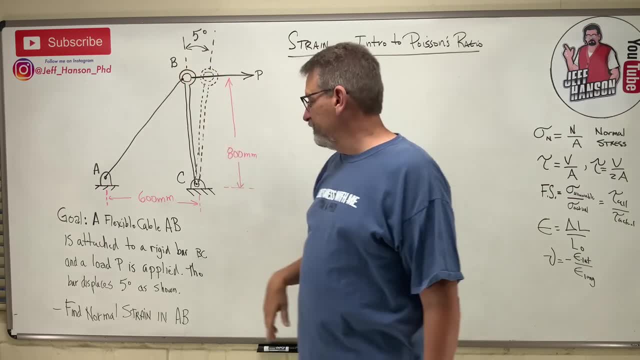 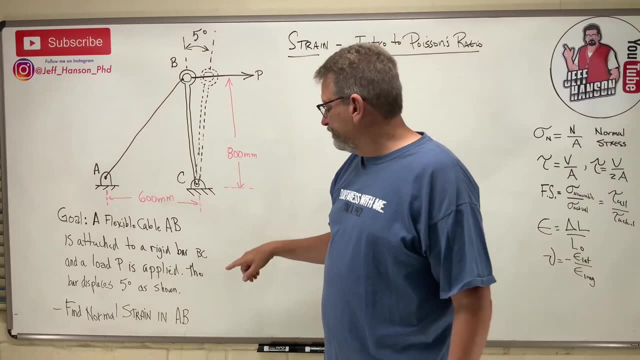 So the dash line is how far that it goes over. So it moves five degrees. Find the normal strain, Normal strain. What does normal mean? Remember that's like along the axis right In the wire AB. Okay, Well, let's. 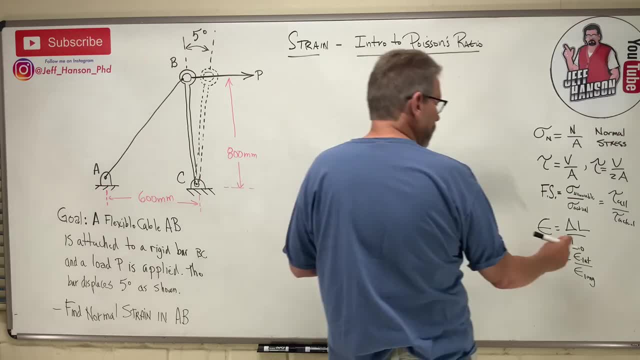 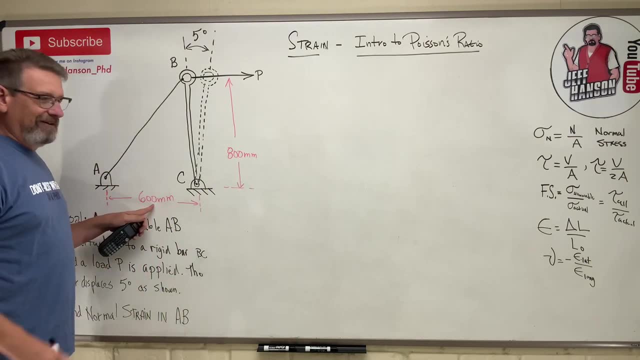 Wait a second, Let's do the before. Let's do before, because we got to have the original length, don't we? The before is here. Hey, look here. Look here, What's 300 times 2?? What's 400 times 2?? 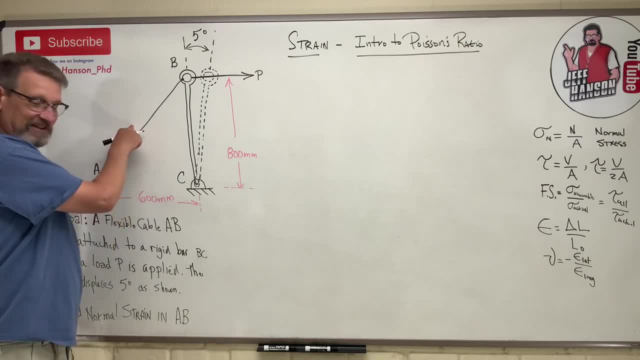 So what's 500?? That's a 3,, 4, 5,, isn't it? This is 1,000,. right, You got to be looking for those 3,, 4, 5s You're going to test. 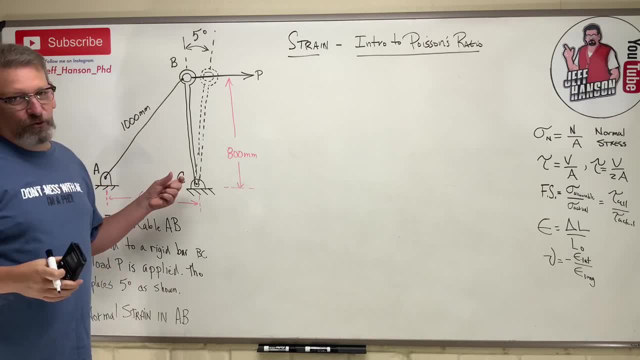 You're trying to go fast. Most of these problems are set up where the angles are pretty easy, But you know, so you need to be able to recognize that. It'll save you a little bit of time, maybe a couple of minutes. 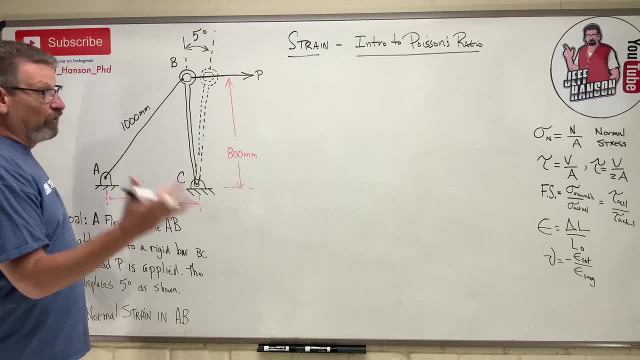 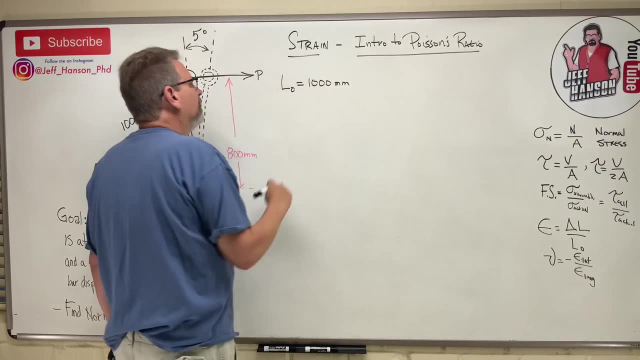 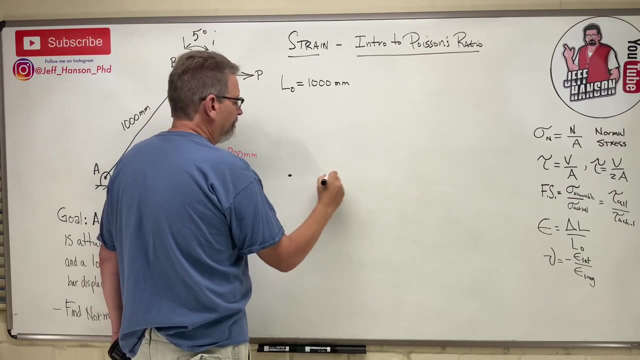 You can work on the next problem, right? Okay, So the original length L naught is equal to 1,000 millimeters. So how long is the cable once it gets stretched? Let's draw it, shall we? 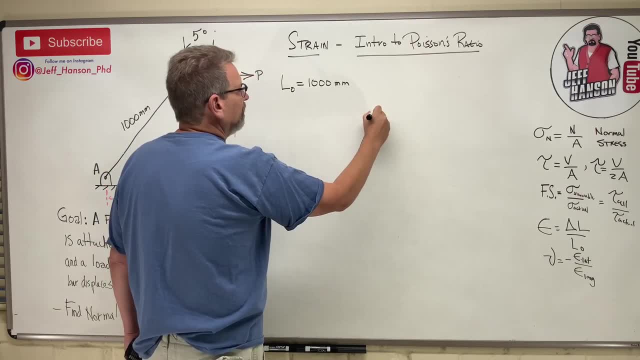 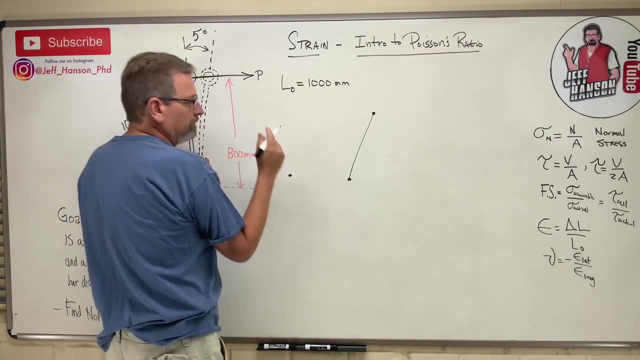 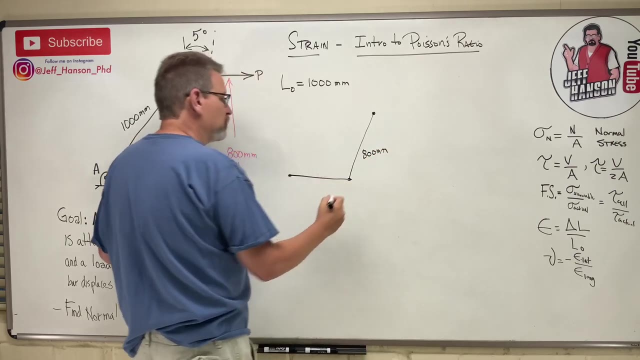 Okay. So here he is, the bar, Okay, And this guy is a rigid bar. So even though it moves 5 degrees, it's still 800 millimeters long, isn't it? Okay? How about this? The distance between these two points down here. 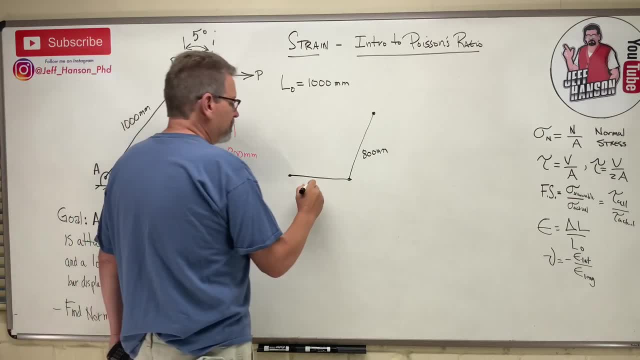 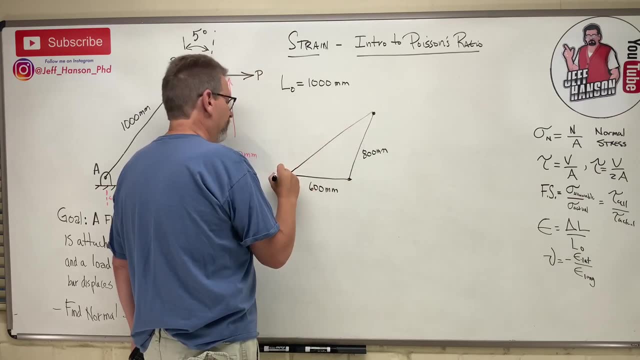 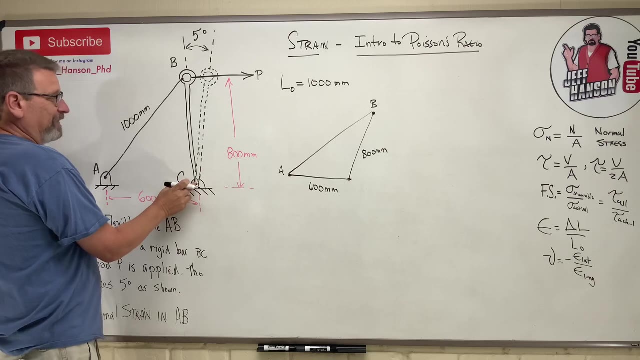 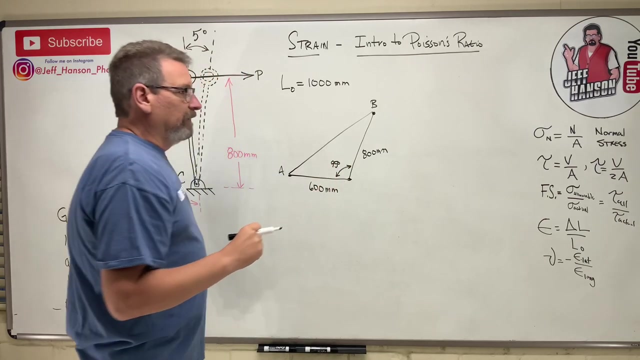 A and C. Does that change? Well, no, So that's still 600.. And then here's the new string, AB. right Here's AB. And what else do we know? This angle right here used to be 90 degrees, but now it's 95 degrees, isn't it? 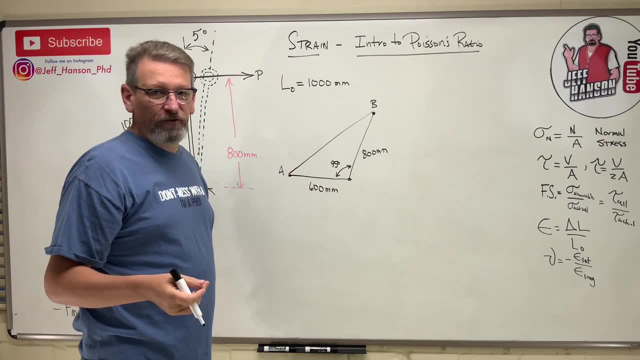 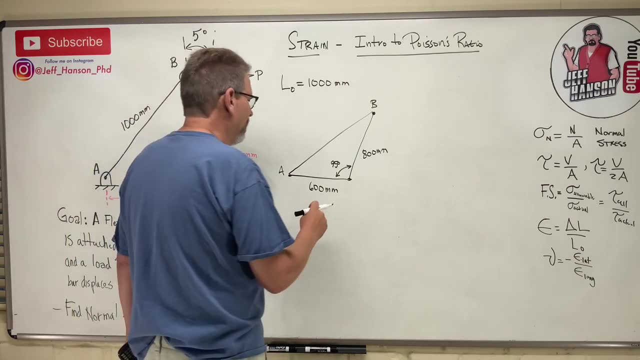 Okay, That's why it's always so hot in the corners. Did you ever notice that in your house, the corners in your house? Because it's 90 degrees. Okay, Never mind, All right, Here we go. So we want to know what is that length right there? 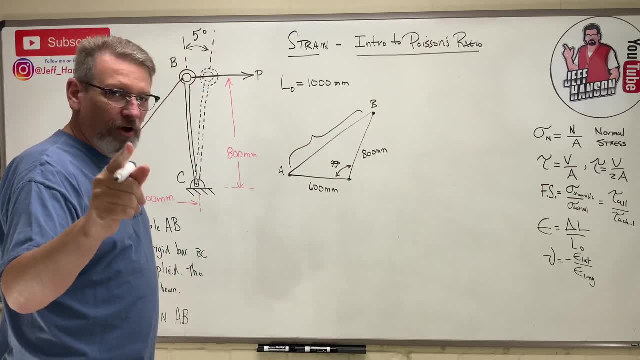 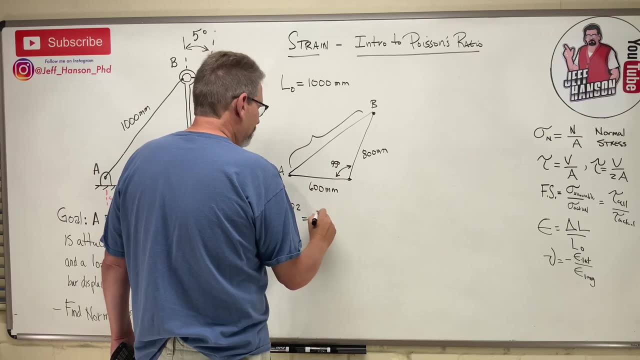 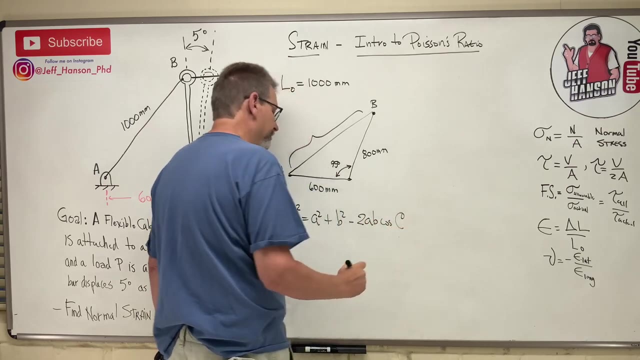 You know what that looks like to me: The law of cosines, Law of cosines Ready, And it goes like this: C squared equals A squared plus B squared minus 2AB cosine of C. Okay, So we got side. 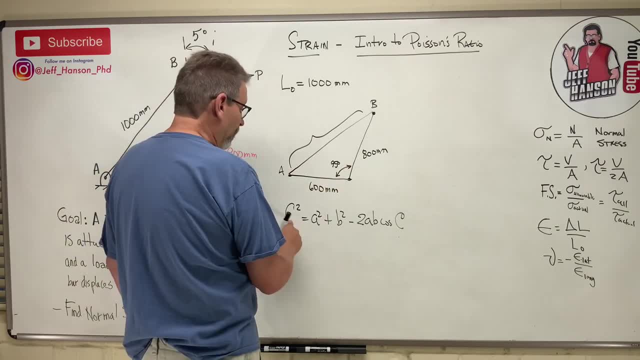 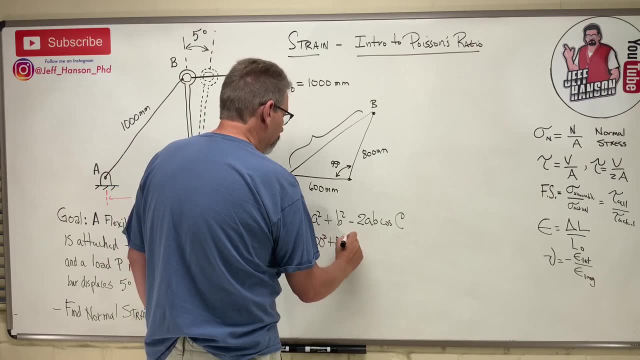 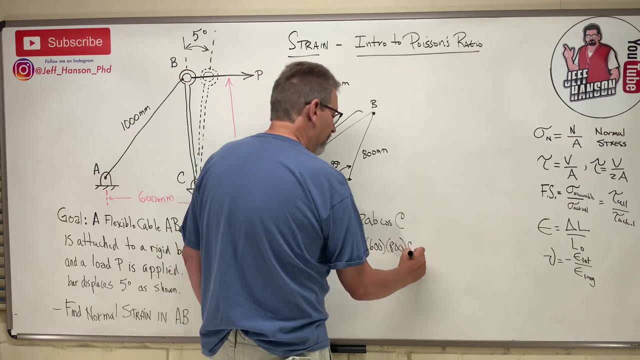 Side angle side. That's what tells me I need to do this right And I'm looking for C. So let's see, That's going to equal 600 squared plus 800 squared, minus 2 times 600 times 800 times the cosine of 95 degrees. 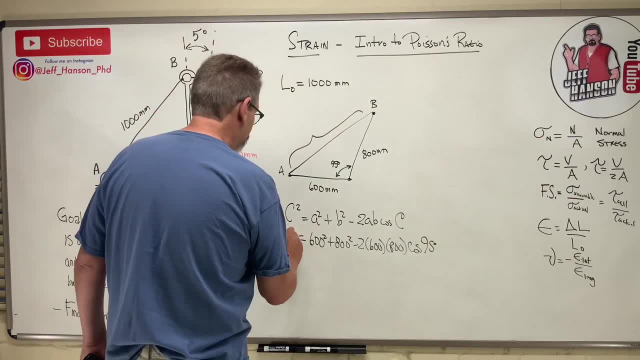 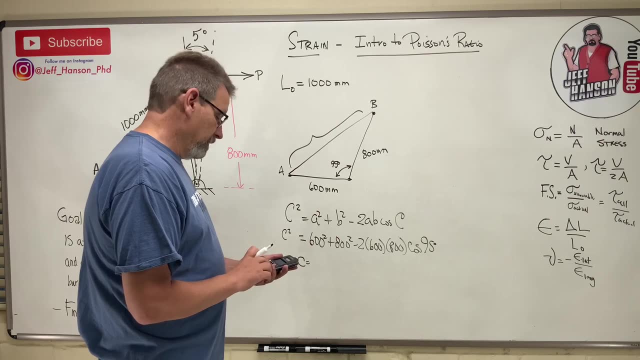 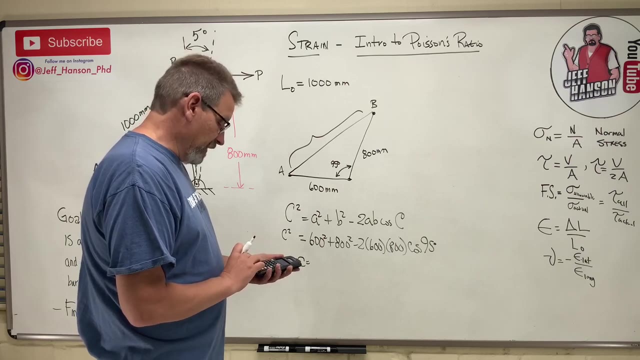 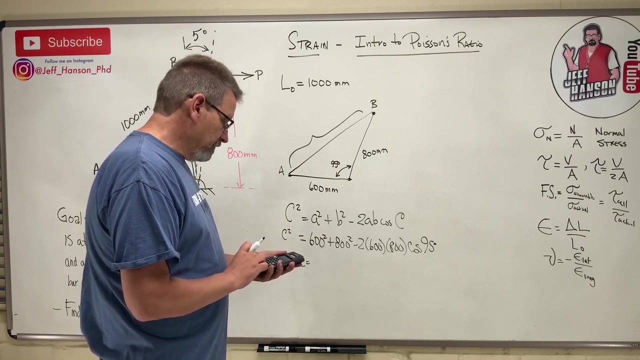 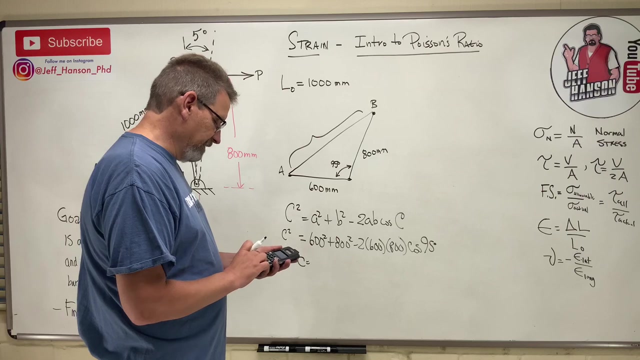 And don't forget, we got to square root this whole thing to get C right. So C is equal to Here we go. All right, Let's see: Clear, Clear, clear, clear, clear, clear. Okay, 600 squared plus 800 squared plus 1200 times, 800 times the cosine of 95 equals: 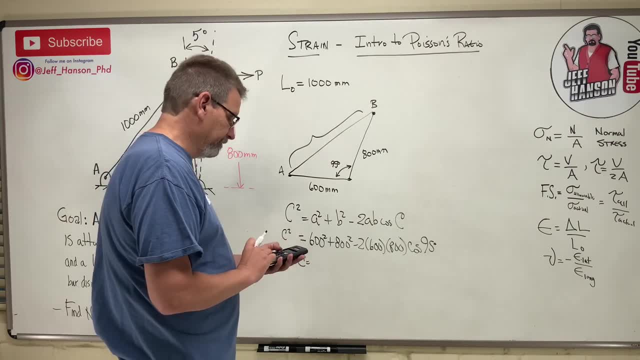 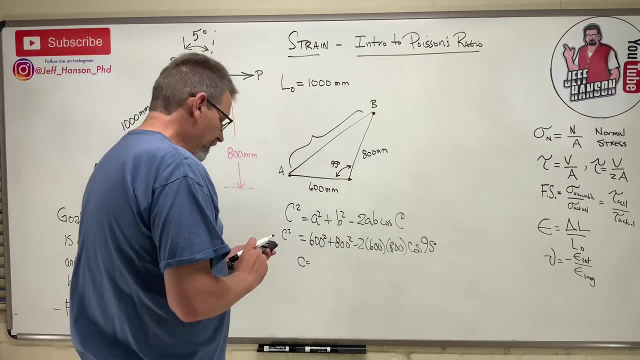 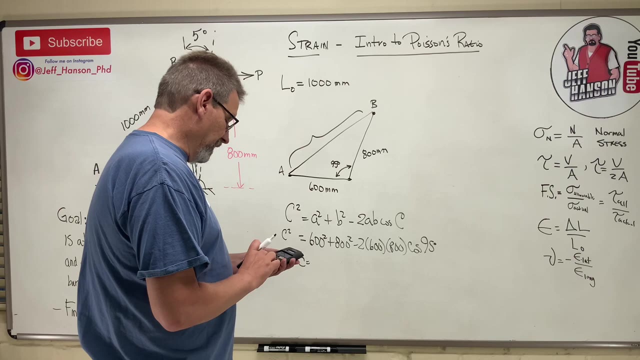 That's a big number, But we got to square root, that, don't we? So C equals No, I got 957.. That can't be right, is it? Let's try it again: 600 squared plus 800 squared, minus 1200 times 800 times the cosine of 95.. 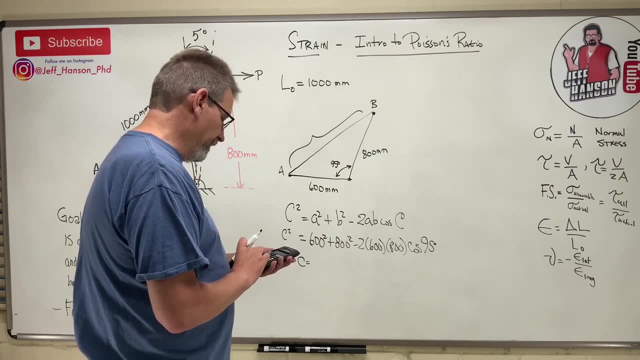 That's a big number, But we got to square root that That's a big number. Okay, So C equals No, I got 957.. That can't be right, is it? Let's try that again: 600 squared plus 800 squared, minus 1200 times, 800 times the cosine of 95.. 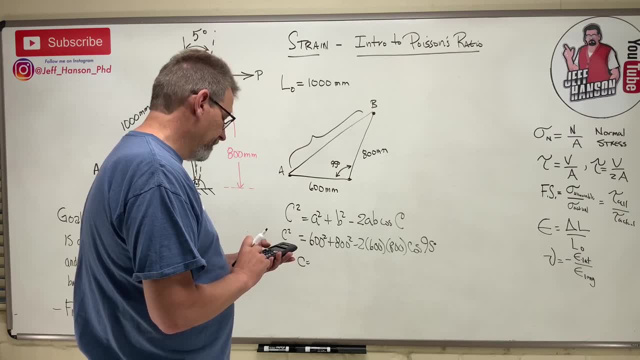 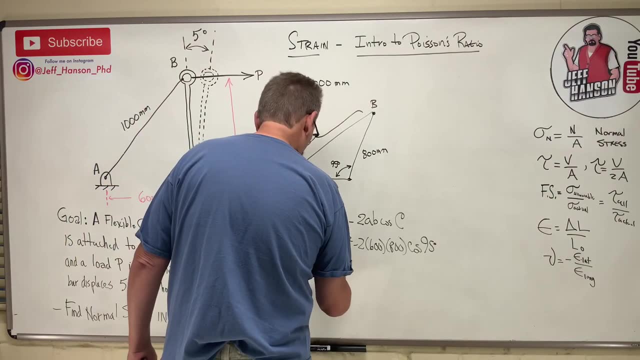 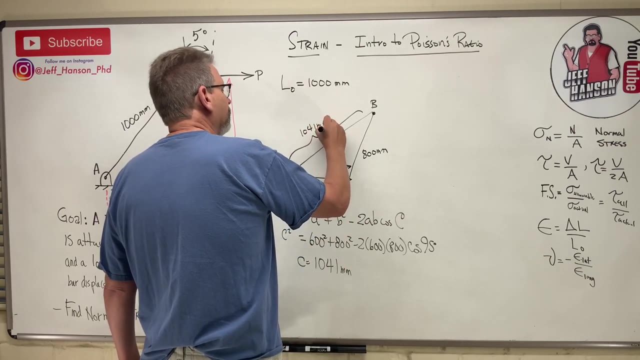 Okay, 600 squared plus 800 equals 1500 times the cosine of 95.. And square root of that, 1041.. Okay, So this guy is 1041 millimeters. all right, So there's our equation, our delta L. Well, he started off at 1000.. 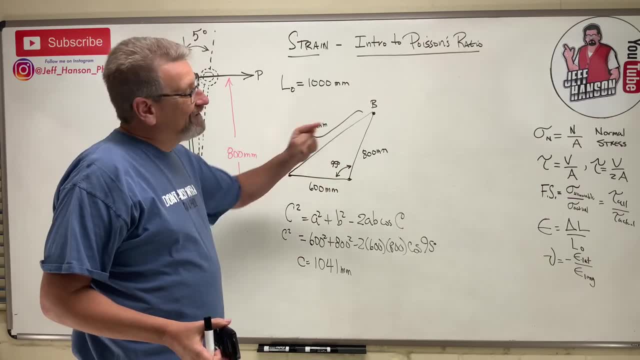 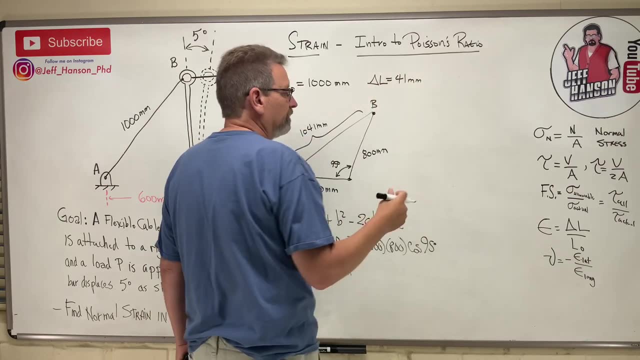 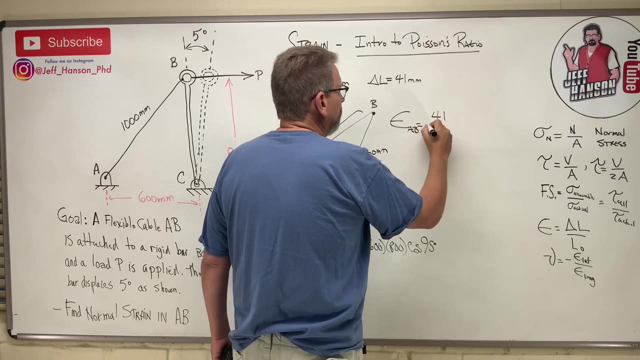 Now how big is he? He's 1041.. So he grew the delta L. Delta L is equal to No, is equal to 41 millimeters, isn't it? so the normal strain in a- b is equal to 41 divided by 1000. 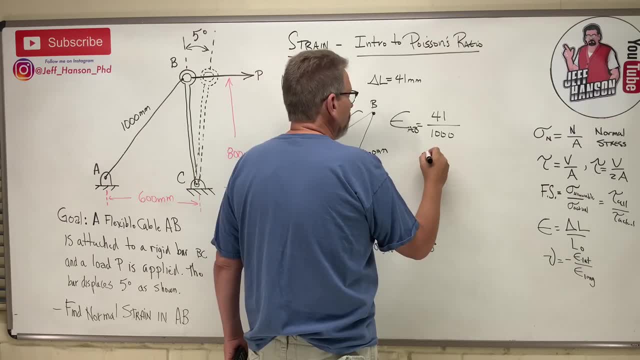 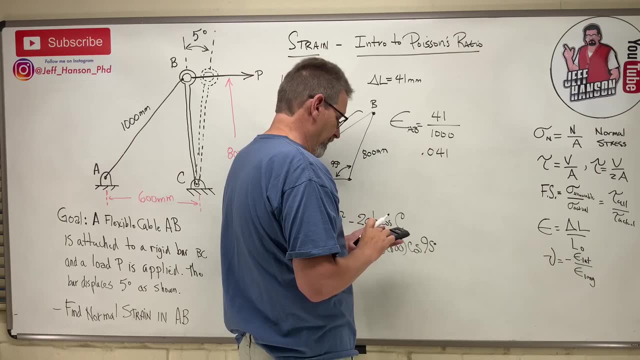 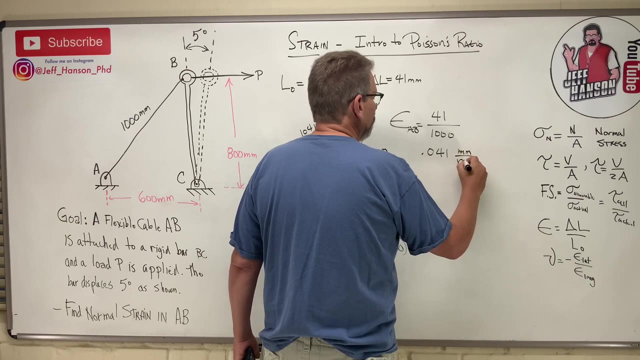 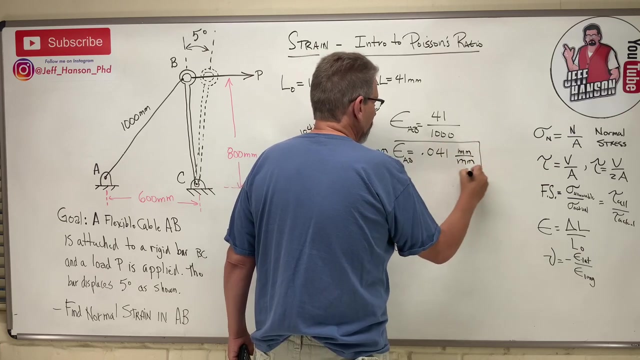 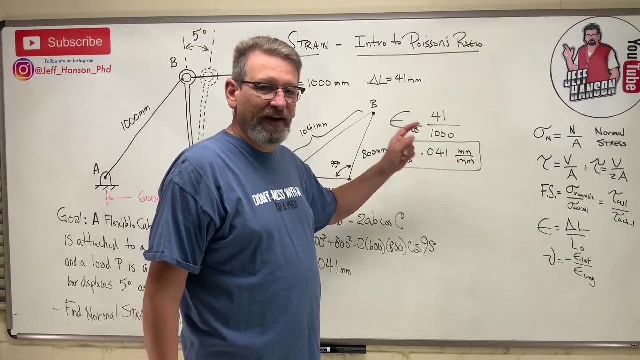 that's going to move my decimal over three places. so 0.041, right, let me do that right. 41 divided by yep, millimeters per millimeter. okay, so that's the strain at for a, b, now that's. so that's, every millimeter is going to stretch. is going to stretch 0.041, now every. 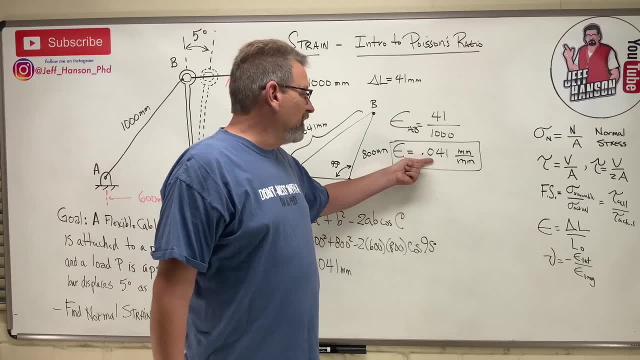 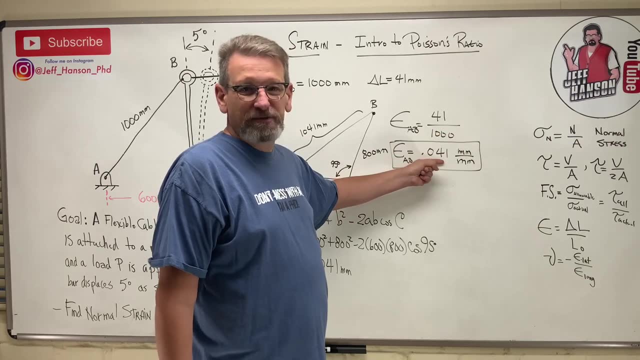 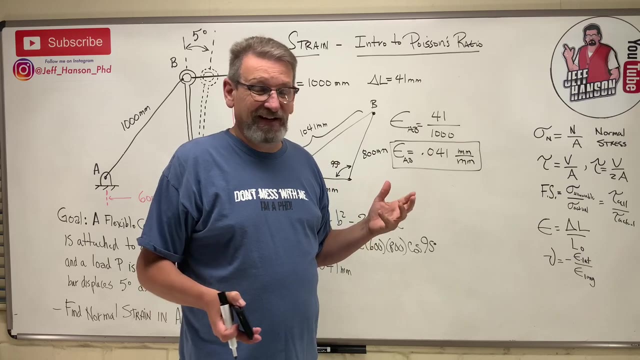 millimeter. millimeter is really little, isn't it? so you're talking about really small numbers here. you're going to have times 10 to the negative, 6 maybe on the, so expect really small numbers for these. strain numbers. right, because steel stretches, but it doesn't stretch like like my little stretchy material did. right, it doesn't stretch like a. 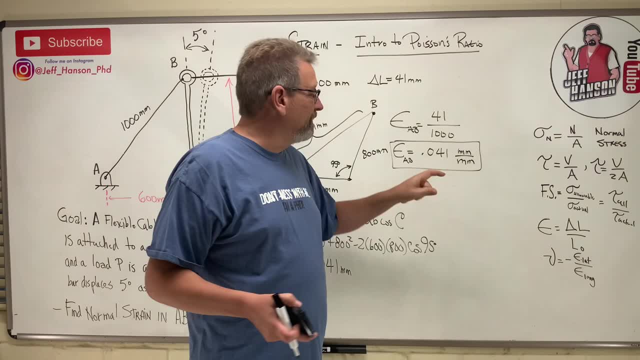 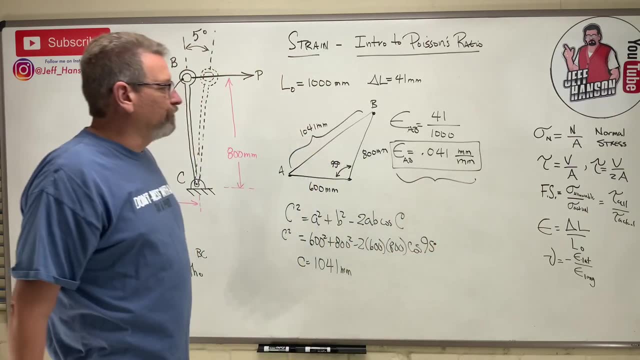 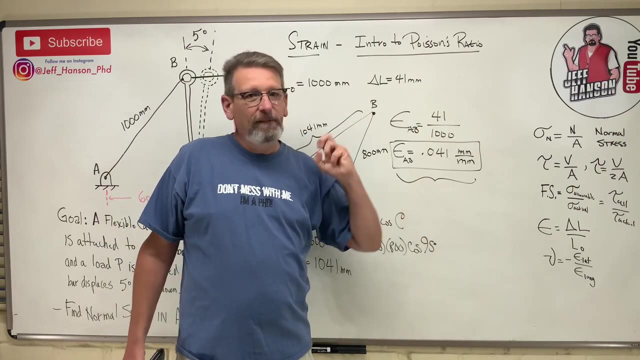 rubber band. it just stretches a little bit right. so these are going to be really small numbers for strain, so you can expect that. so there's a good little introduction to strain problems and a little introduction to what the heck is poisson's ratio. now you know physically what. 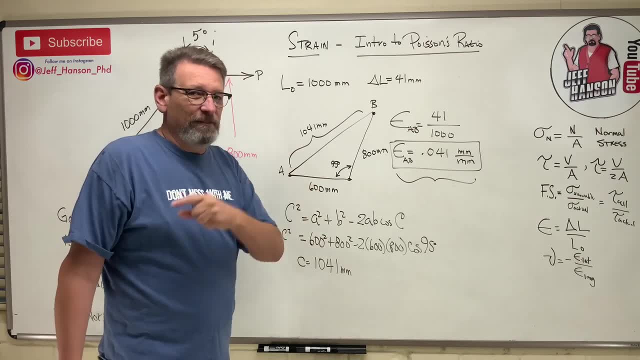 poisson's ratio is what it means, and now, when you come to the next problem, we'll know how to use it. so i'll see you on the next problem.